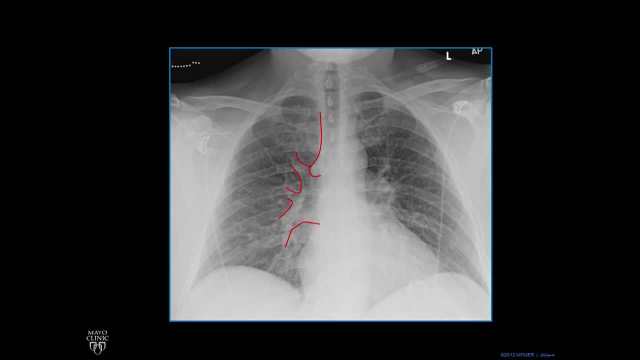 radiograph and we're going to look at the pulmonary x-ray And we're going to look at arteries and the pulmonary veins together. we're also going to look at the right atrium, this contour, which is the left subclavian artery, the aortic arch. 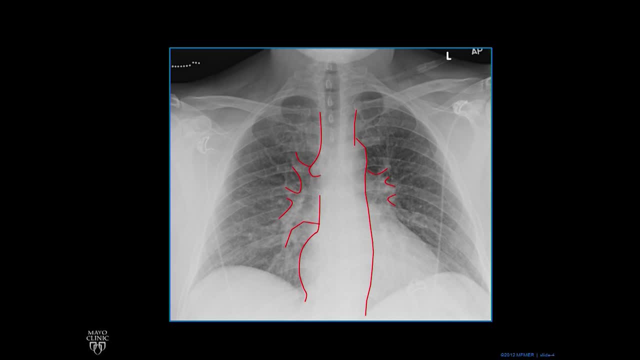 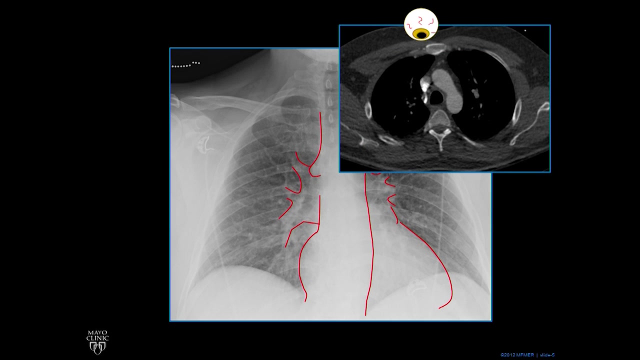 and the descending thoracic aorta, the hyla on the left, which in this case is mostly pulmonary arteries on the left left atrial appendage and the left ventricle. so there's our eye in the sky looking from the front, and we can see. 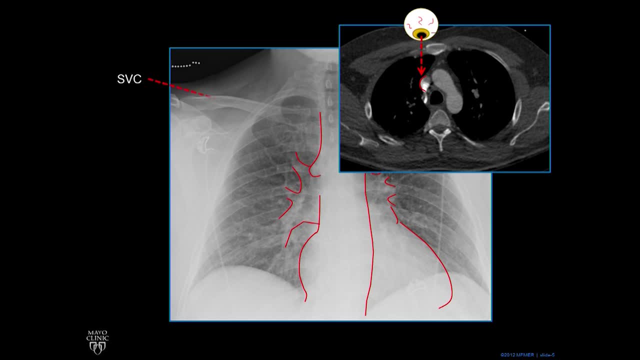 that bump and the reason you can see this bump, which is this case, is the superior vena cava. the SVC is if there's a tissue air interface. when you're looking from the front and frontal radiograph you'll see the structure. so in this case the SVC bumps against lung and so it shows up as a, as a line which 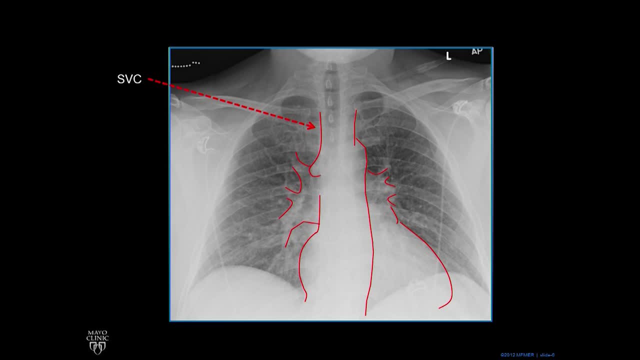 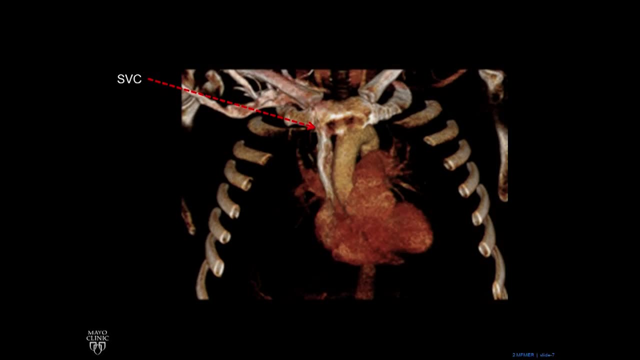 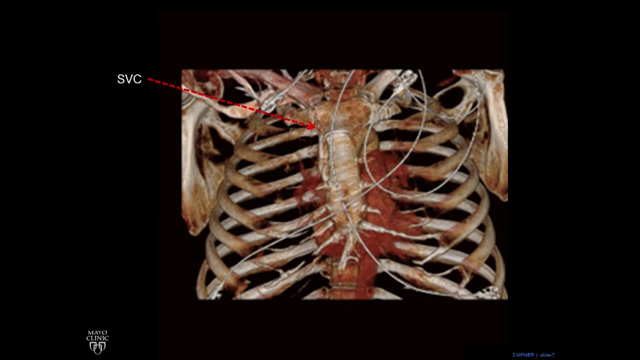 you can see this here, look. so here's our chest x-ray, and then we're going to fade it out and we overlay a CT scan, a 3d volume rendered CT scan from the same patient and you can see that that line really is the superior vena cava. it drains down. 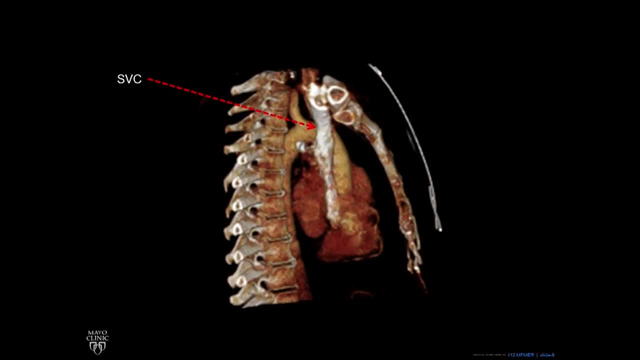 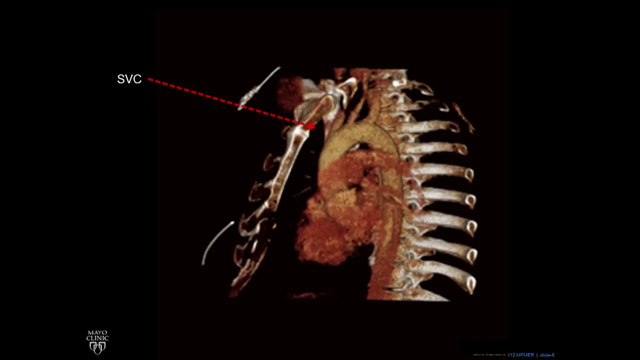 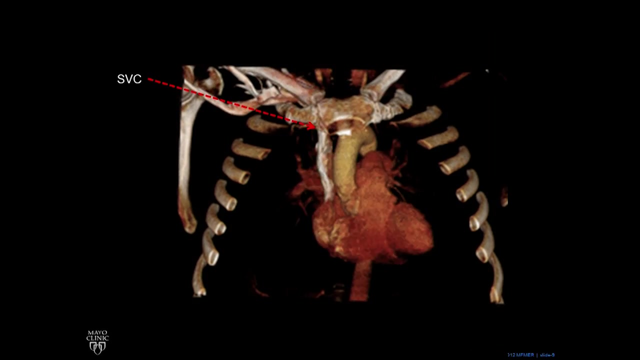 into the right atrium. we rotate it around and you can see the superior vena cava draining into the right atrium. we spin around from the back. you can also the SVC from the back, which we'll get back to. and there we are and back to our radiograph. 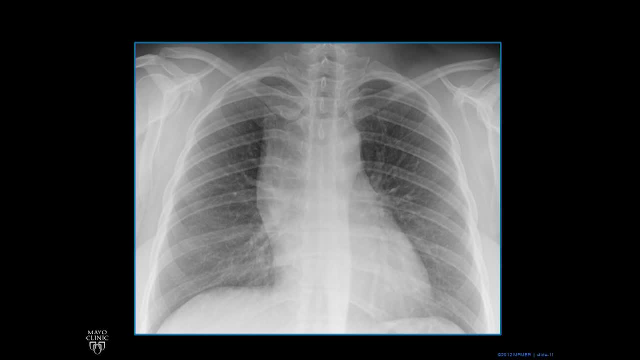 so look at this case. this is not normal. what is this abnormal contour? in most cases, an abnormal contour in this spot would have to do with adenopathy or some sort of mass, but because the point of this talk is to show that that contour really is the SVC, we'll show this case. so 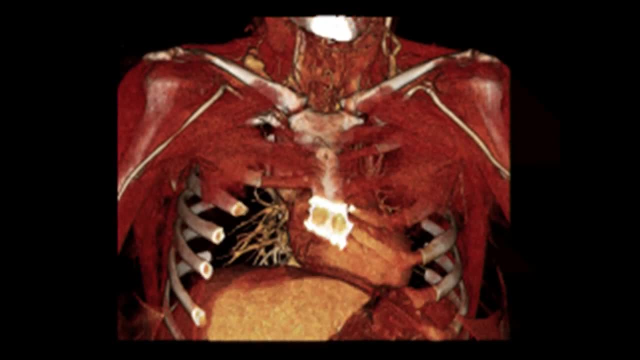 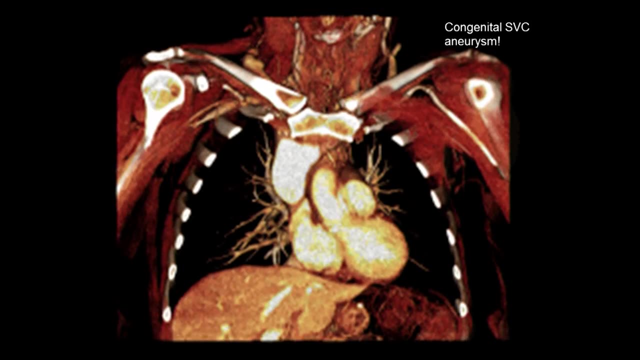 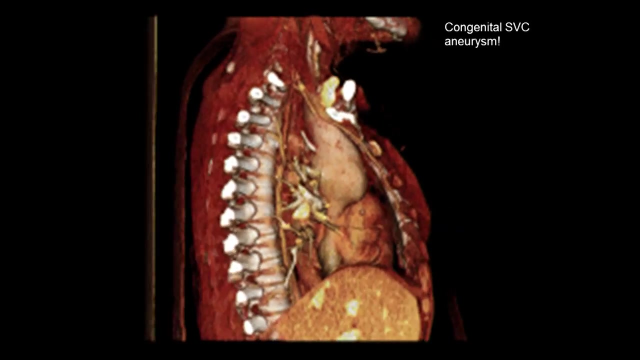 we fade away, we overlay our CT scan, we peel back, we peel back. and what is that? this is a congenital SVC. aneurysm is in a young woman in her 20s or 30s. not sure why she got that, but you can see that that big structure is the SVC. we're rotating around, we're looking from the back. 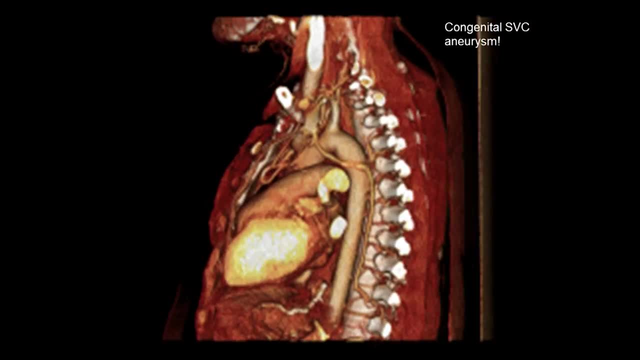 we see the DCF. we're looking from the back. we're looking from the front. we're looking from the back. we see the DCF. we're looking from the front. we're looking from the back. we see the DCF. we're sitting. thoracic aorta. now we can see the left ventricle and the pulmonary. 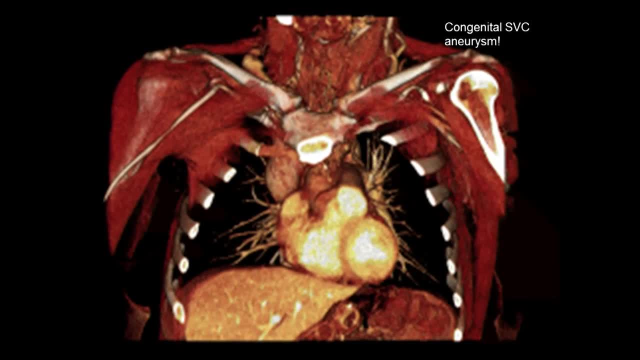 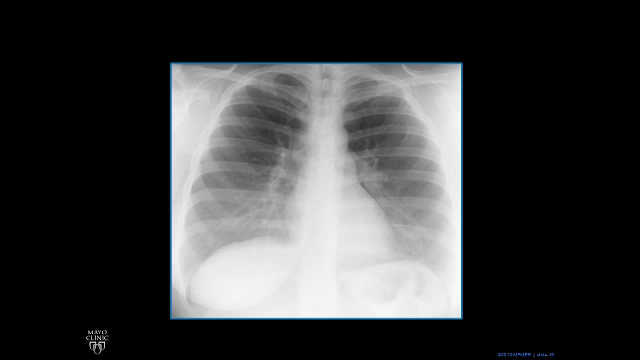 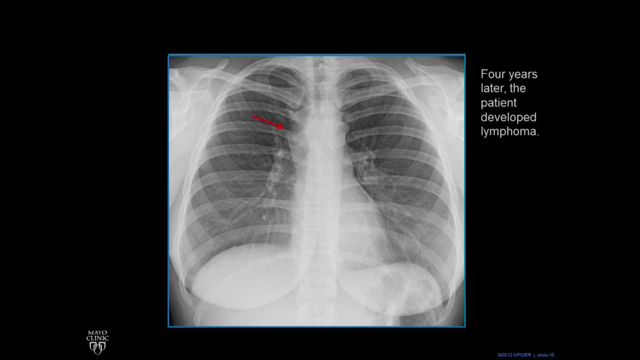 arteries and we come back to the front and there's our big SVC, right where it's supposed to be like this. this is a normal chest x-ray. however, four years later this patient developed lymphoma. now, in the region of the SVC there's an abnormal contour, there's too much soft tissue. you can see with that red arrow. 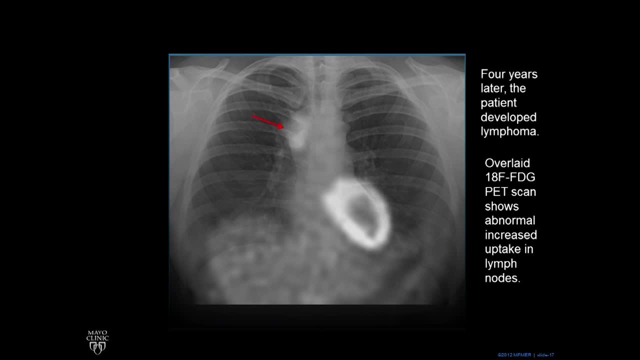 we overlay an 18 f fdg pet scan which goes to areas of increased metabolism. so in this case that mass is lighting up because it's using more glucose than usual. it's a lymphoma and the left ventricle, which is the other region, down. 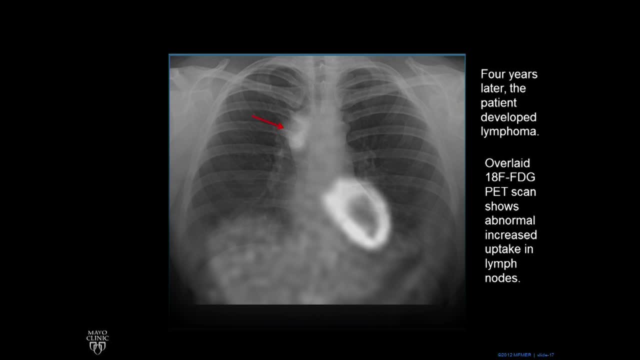 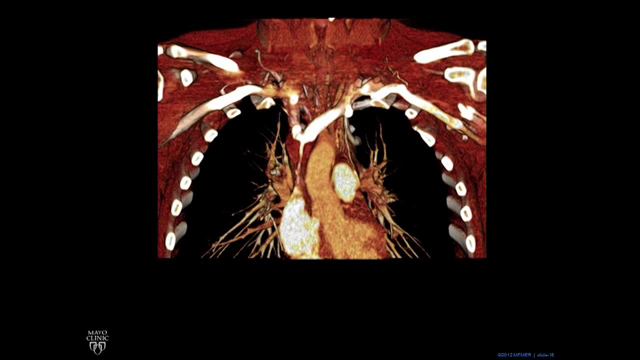 there lights up because that's normal, so you can see increased uptake in the lymph node in that region that Abner will contour. there is a mass. we peel away to the CT scan and you can see that there's an abnormal red dot in there on the upper part of the轉. 我是 فيoy持JOь Edward. 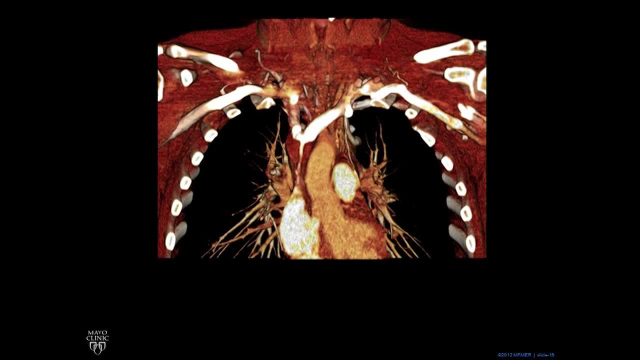 there's mass encasing the superior vena cava. the brachycephalic veins, which are the veins which drain into the vena cava, are dilated and there are numerous collaterals veins draining the upper body into the lower body venous system. so all these veins are abnormal. they're trying to. 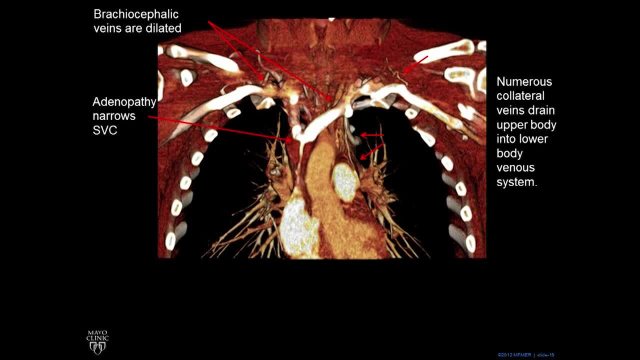 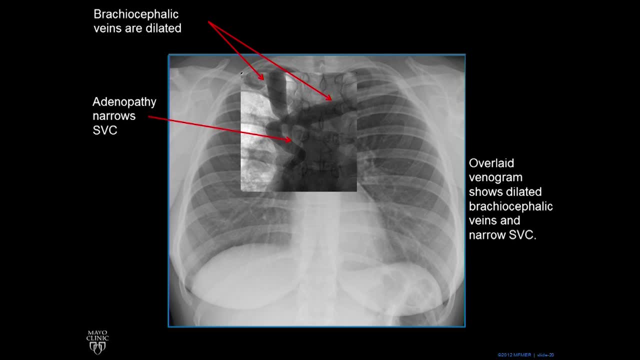 bypass the SVC and get to drain the upper body into the lower body and you see, we go back to the radiograph. we overlay an angiogram. these are injections from veins in the arms and you can see that the brachycephalic veins here are dilated and this arrow points to a little skinny. 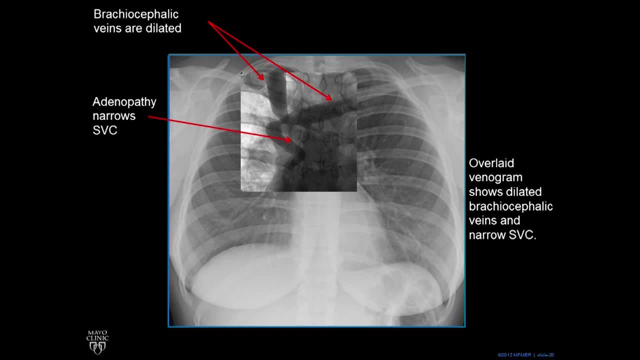 line, not the swirly s on the front, but and skinny line be hacked behind. that's the narrow superior vena cava. this dilated squiggle in front is an internal mammary vein which acts as a collateral lens out anterior. the narrow one is the superior vena cava. 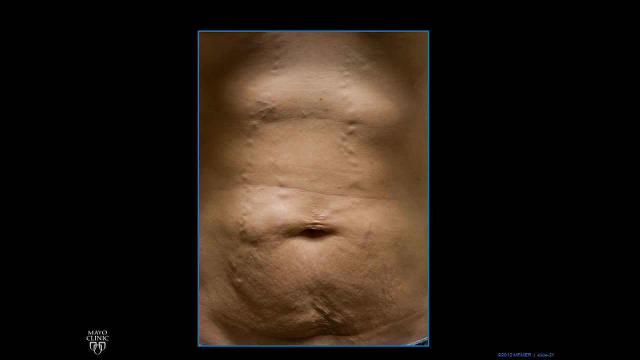 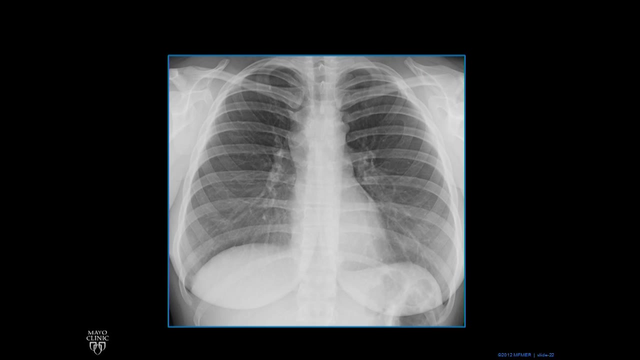 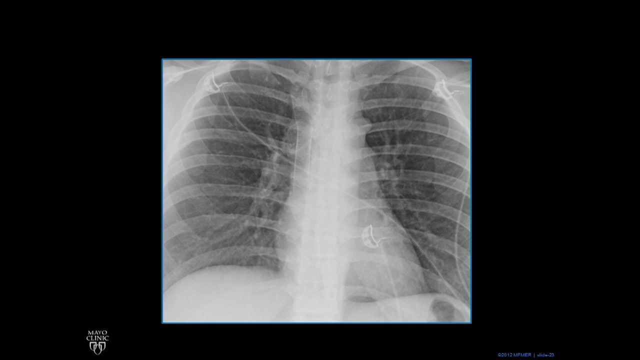 this patient had collateral veins that you could see on their abdomen as the varices, and all these veins are trying to drain from the head to the body. so what happened? a stent was placed there to open up that superior vena cava and relieve the obstruction. the person was getting plethora.